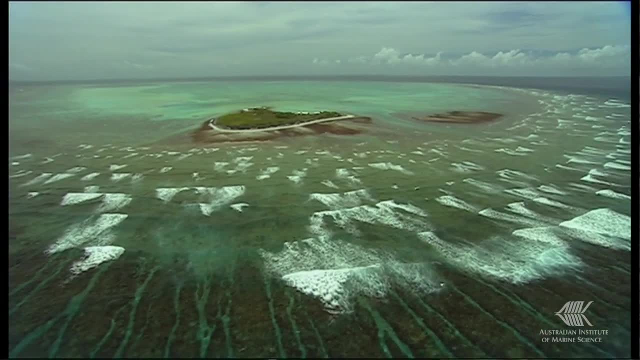 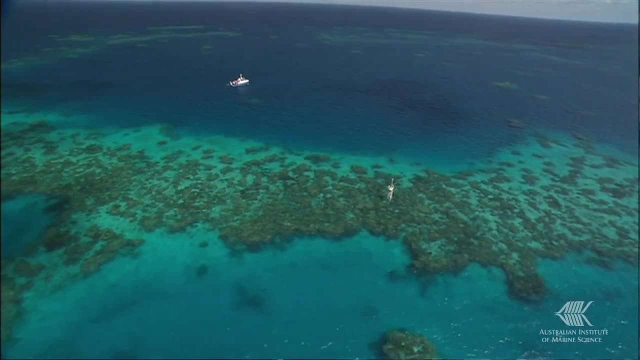 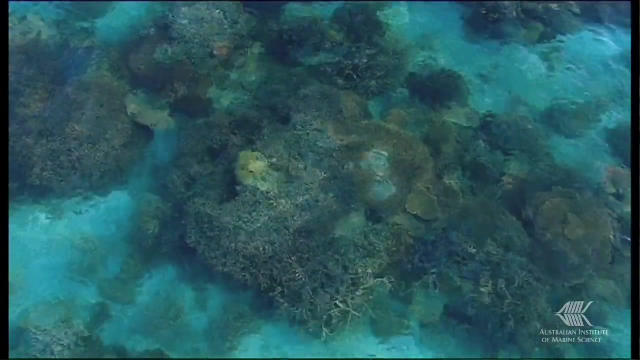 balance between reef construction and destruction is now under ocean acidification: a one second difference: One step forward, two steps backwards process. The consequences of this can be severe, as it means that reefs will be unable to repair themselves after storm damage. It also means 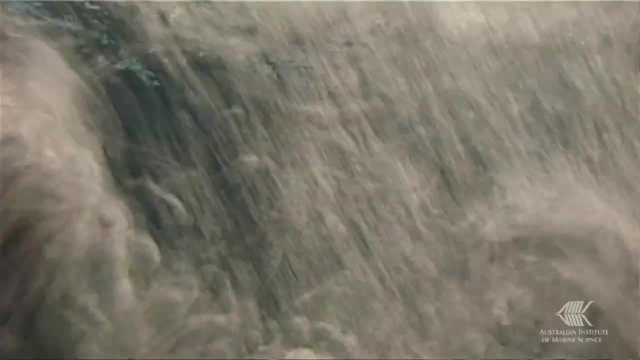 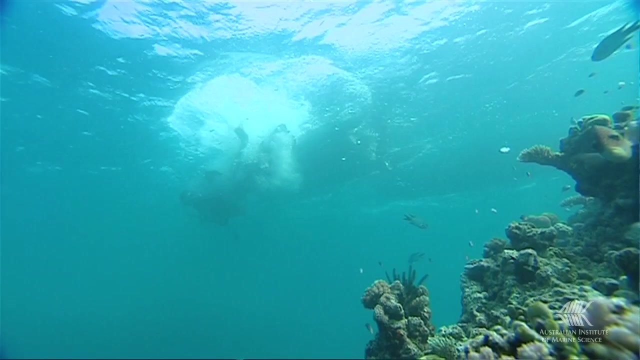 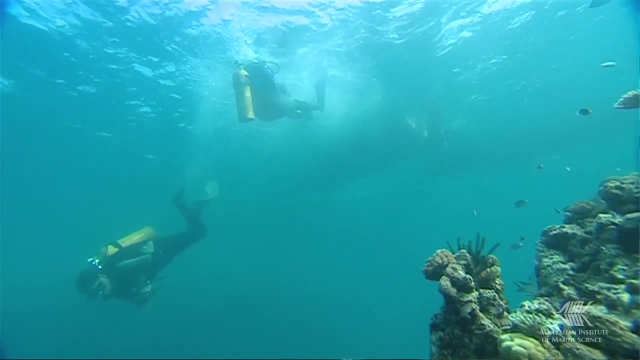 that reefs will have less structure, and with less structure they have less habitats for fish. Finally, reefs may not be able to keep up with sea level rise under ocean acidification, And just imagine what that means for island communities in the Pacific. 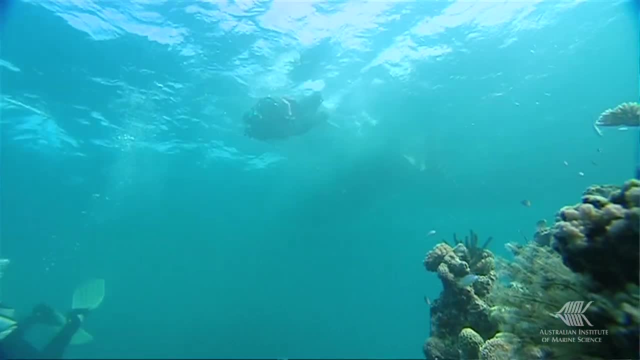 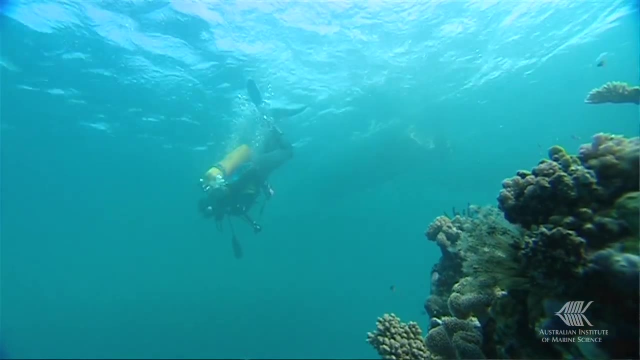 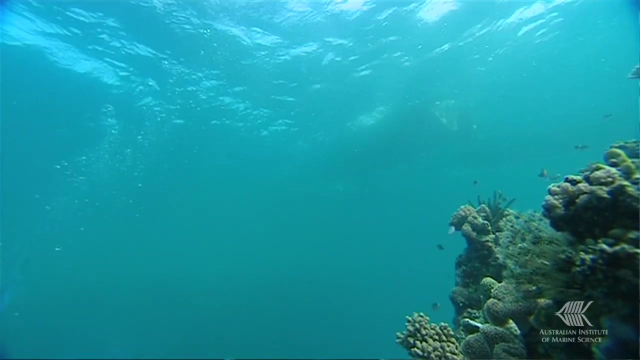 That ocean acidification has been regarded as a quite uniform threat, with risks to all coral reef areas globally being equal. What we have found in this study is that some coral reef areas, in fact, can modify their own pH, some in a positive way and some in a negative way. This really comes down to 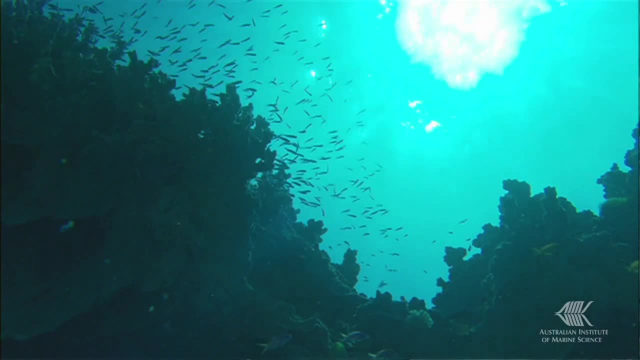 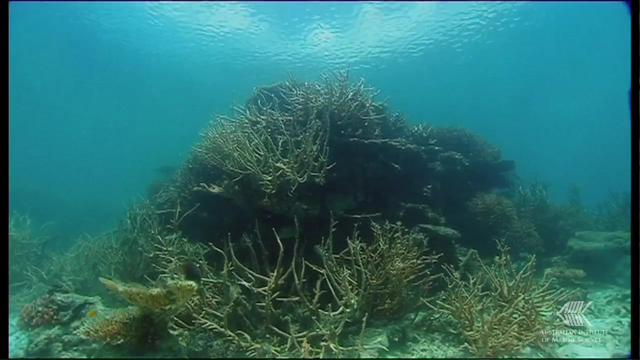 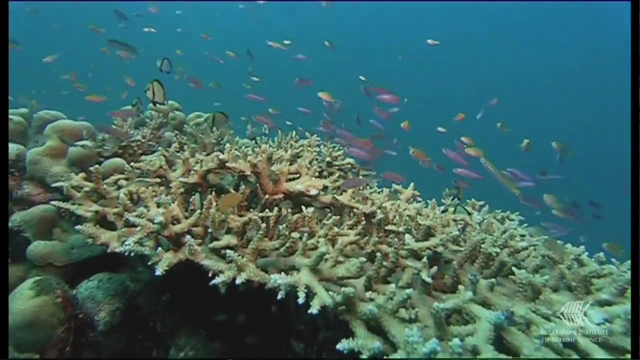 the biology of the reef organisms themselves. Now, as you know, coral reefs are made up of organisms that respire just like us, so they produce CO2 themselves, which locally can add to the problem. But many reef organisms also photosynthesize like plants, so they take up CO2, which reduces the effects of ocean acidification. What we have found in this study is that areas with high rates of photosynthesis, such as seagrass beds and lagoon areas with sand and algae, can make coral reefs next door, so their neighbors, less vulnerable to ocean acidification. 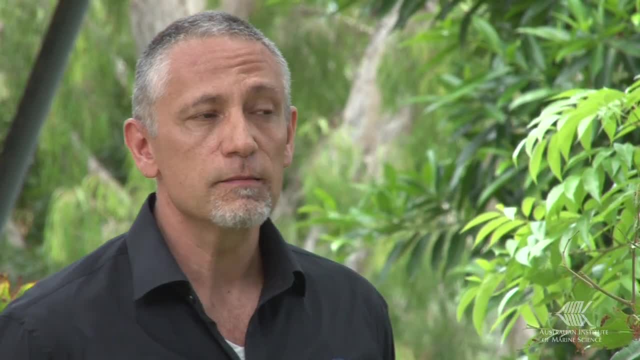 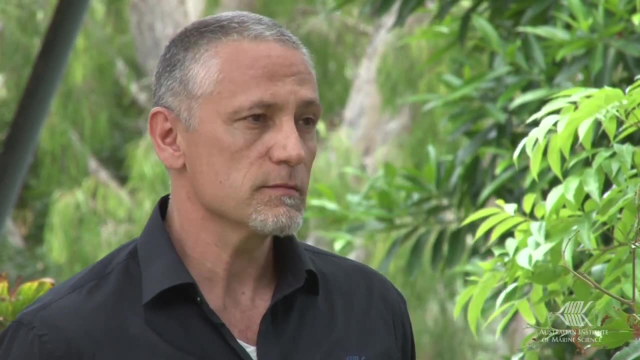 What this study can do is help us better understand what reef areas are capable of and what they can do to reduce the risk of acidification. This is a big step forward, as managers and policy makers have previously assumed that all reef areas have equal risk. 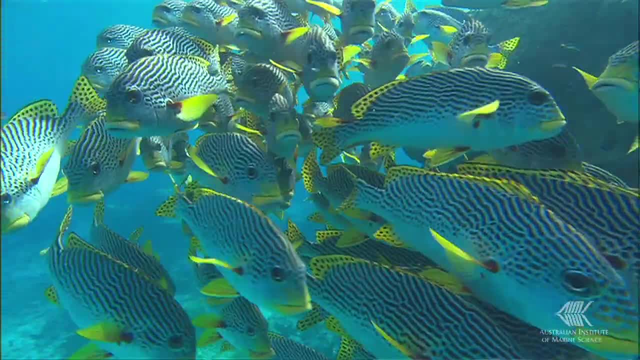 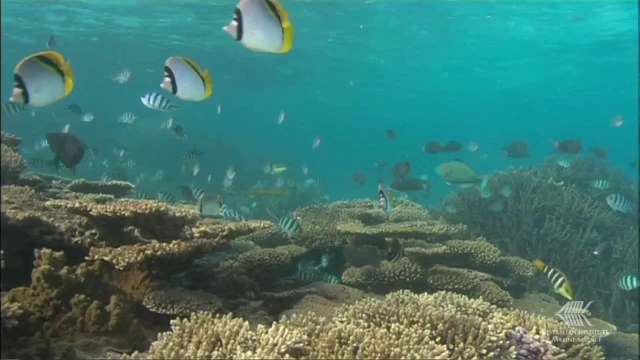 This can help us better plan for the reef's future. It can help us understand how different natural reef habitats can help each other reduce the risk of acidification and where we need to intensify our care and our management. For example, if we can promote a healthy seagrass bed area in a reef, we can reduce the risk. 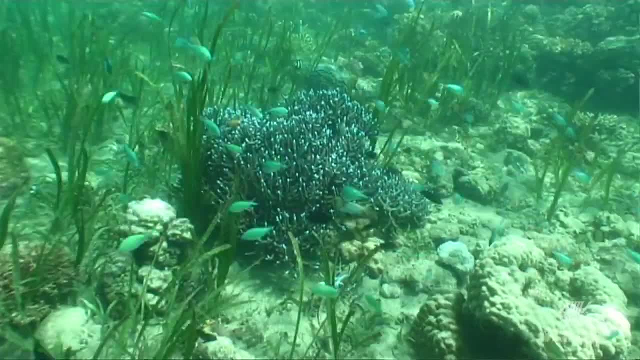 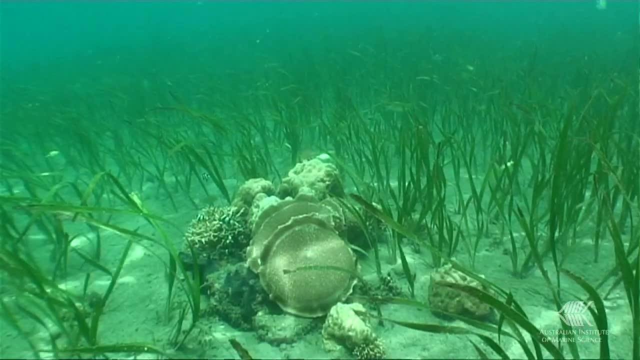 of acidification. For example, if we can promote healthy seagrass areas in a reef, we can reduce the risk of acidification. We may be able to give critical or high-priority coral reef areas a helping hand. In other words, we may be able to buy those reef areas some time until we can tackle the. global threat of ocean acidification and climate change by lowering carbon emissions. 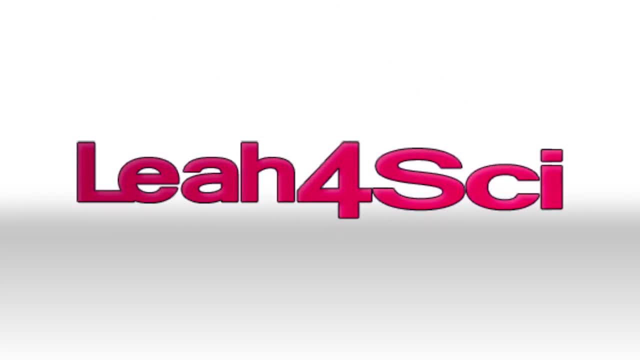 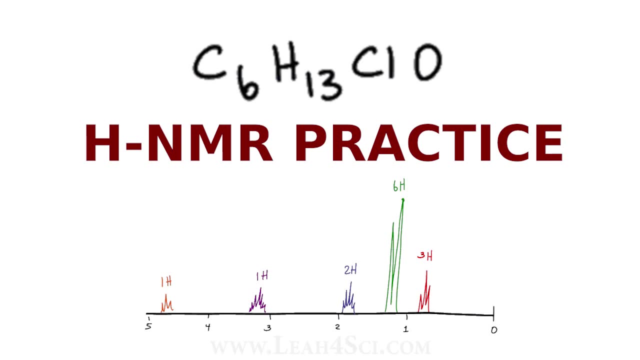 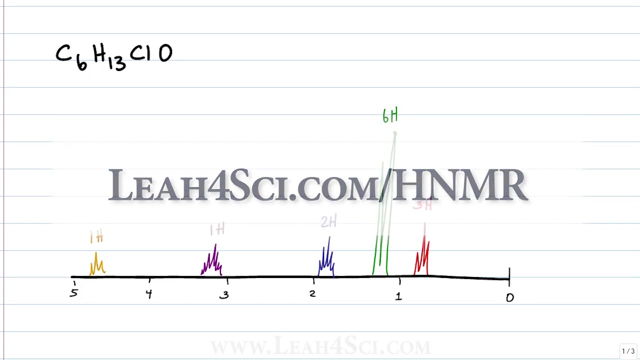 Leah here from leah4scicom, and in this video I'm going to show you how to solve for the molecular structure when you're given a molecular formula and an HNMR graph. You can find this entire video series by visiting my website, leah4scicom. slash HNMR. The first thing to